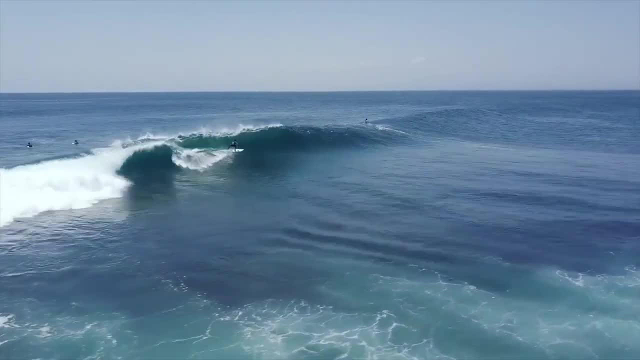 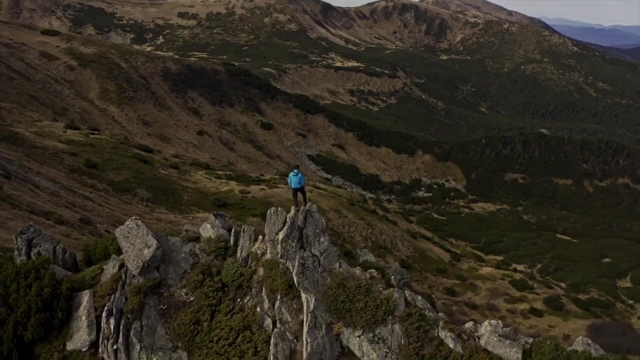 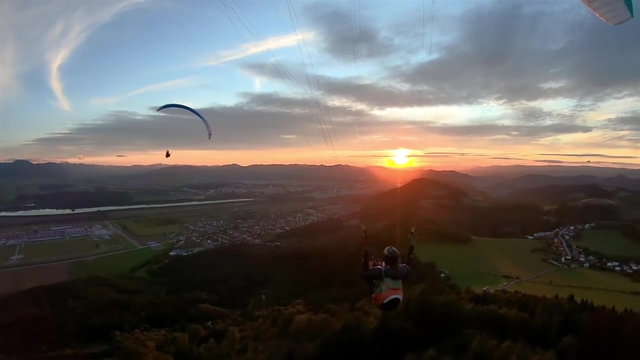 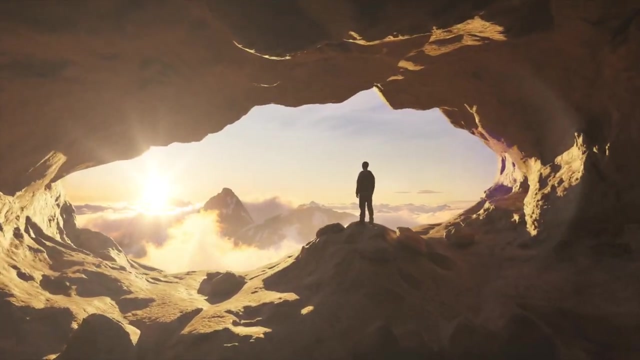 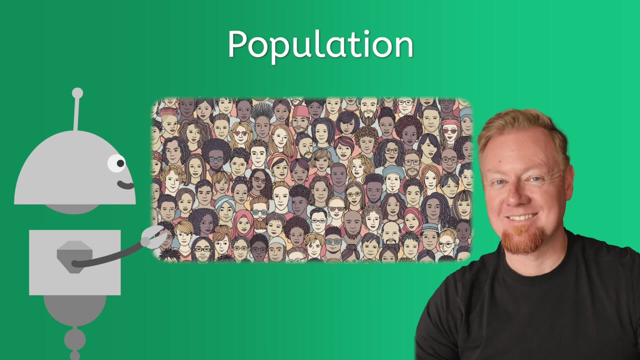 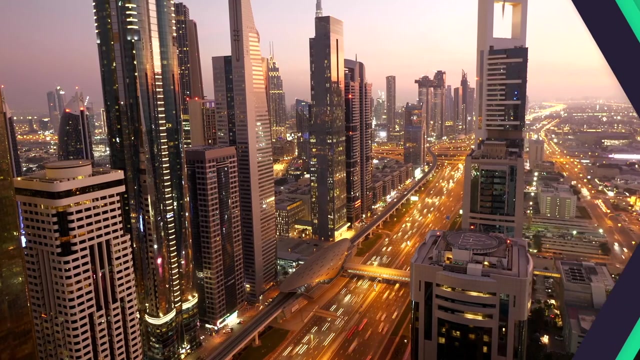 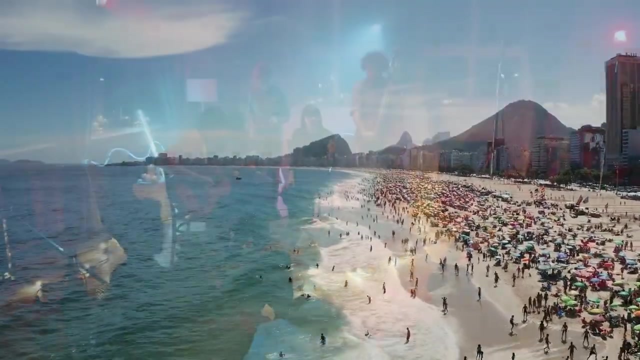 Hey there, Explorers, Brian here. Now that we've made it through our geology mini-unit, it's finally time to start talking about populations. Now I know what you may be thinking: Population, You mean people. Why is there a whole separate lesson on that? Aren't we going to be talking? 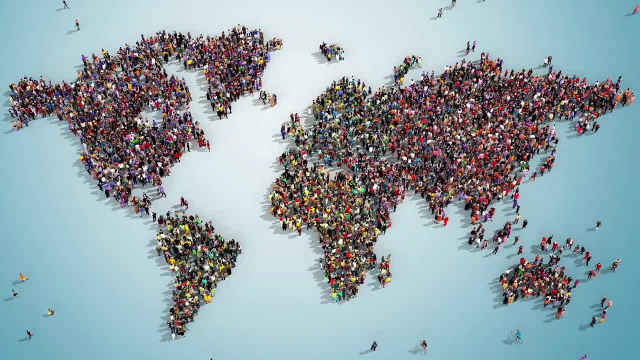 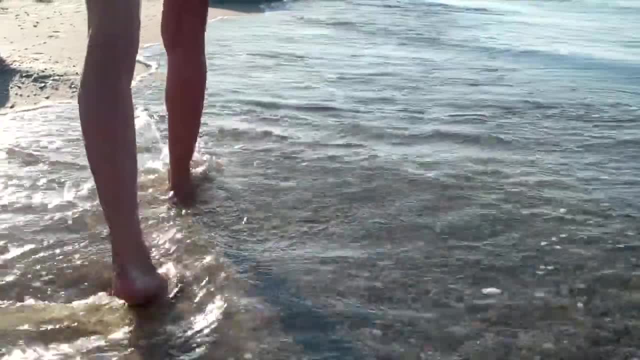 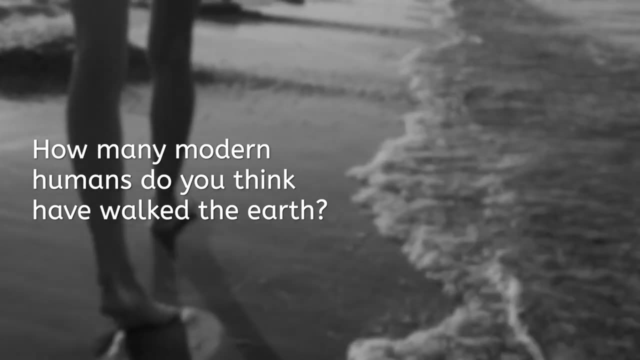 about people all year. We can't be trying to talk about like all the people at once, can we? That's a great question, and so let me answer with another question: How many people do you think have ever walked the Earth? In fact, record a response and 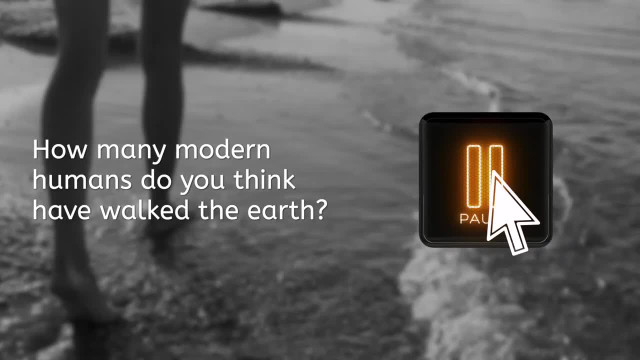 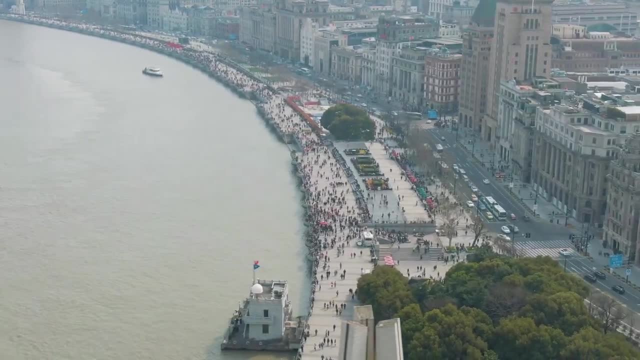 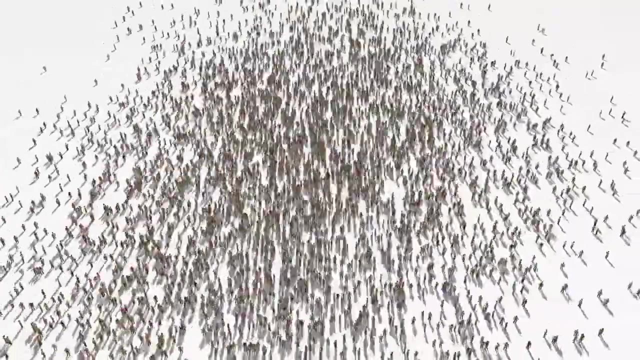 explain your reasoning in the lesson guide. The most reliable estimates are between 90 to 110 billion people. That may sound like a lot, but let's do some simple math. The current population is around 7.9 billion people, So somewhere between 6 to 10% of all people. 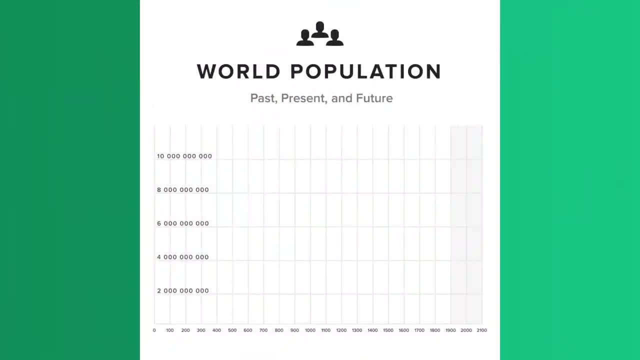 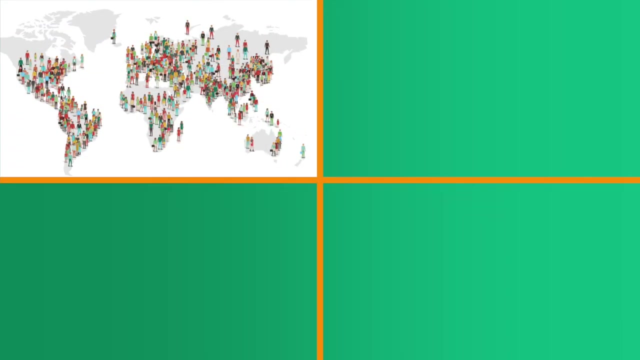 who have ever lived are alive. The sheer number of humans living today makes the world a very different place than it was just 100 years ago. As the world's population has grown, patterns of human settlement have changed with it: Measuring where people live, how many people live there and why they live. 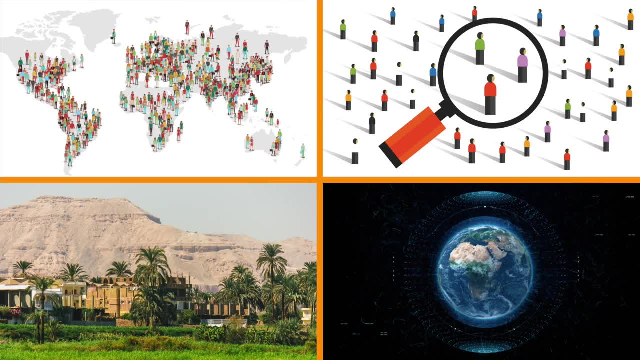 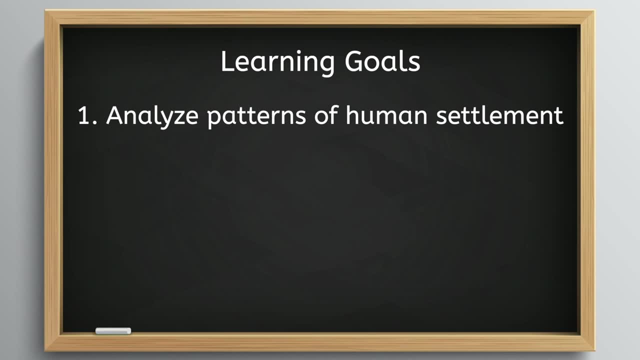 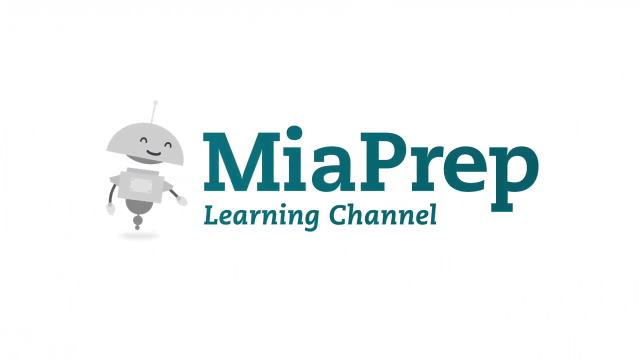 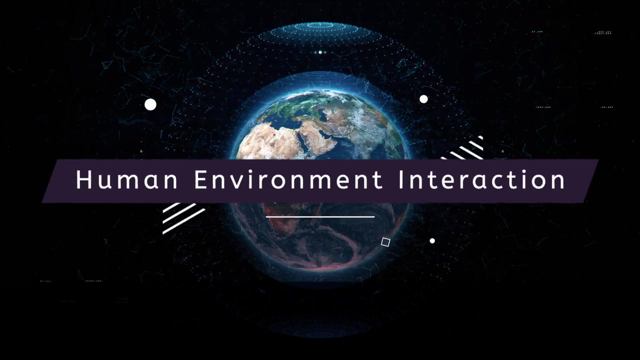 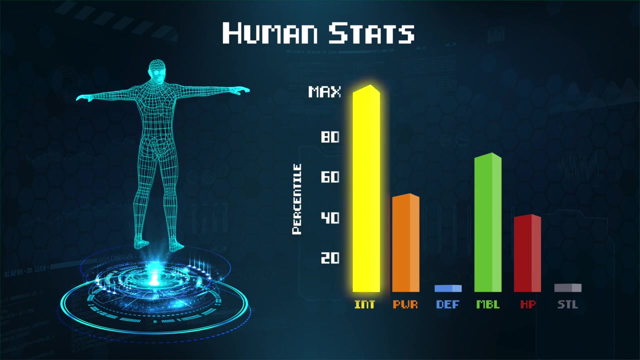 where they do, can give us invaluable geographic information about our world. Our learning goal for the day is to analyze patterns of human settlement. To do this, we'll examine population distribution, density and composition. Ready explorers. One of the premier hallmarks of humans is their ability to adapt. As a result, humans 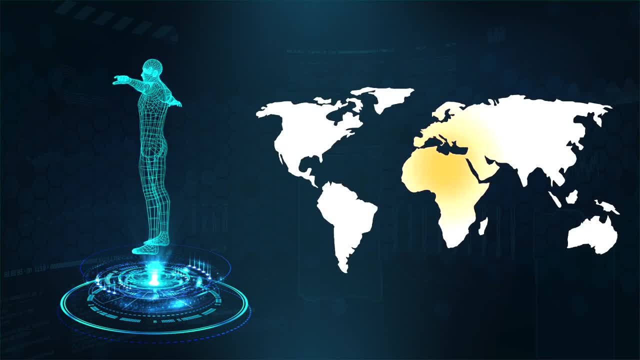 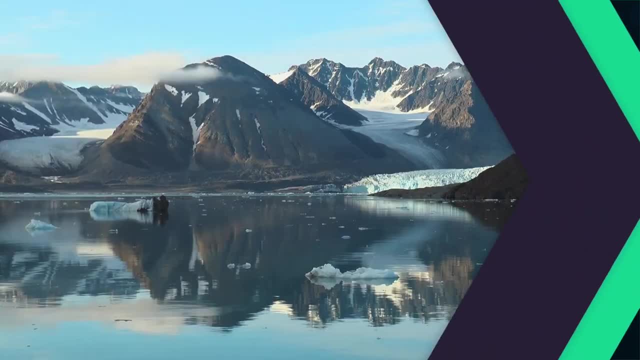 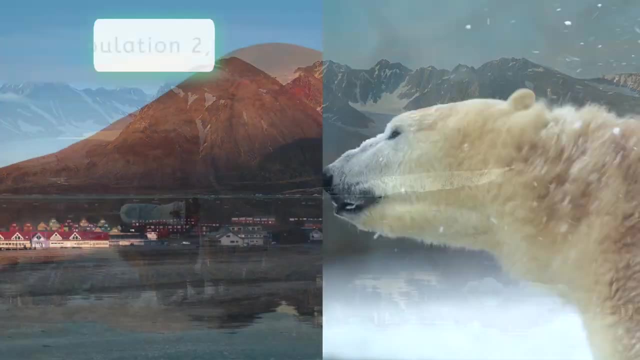 have spread to every corner of the Earth. You can find humans on every continent and in many places which might be considered inhospitable. The people of Svalbard, Norway, have three solid months of sunlight and then three solid months of twilight, And the 2,000 people living there share the space with over 2,500 polar. 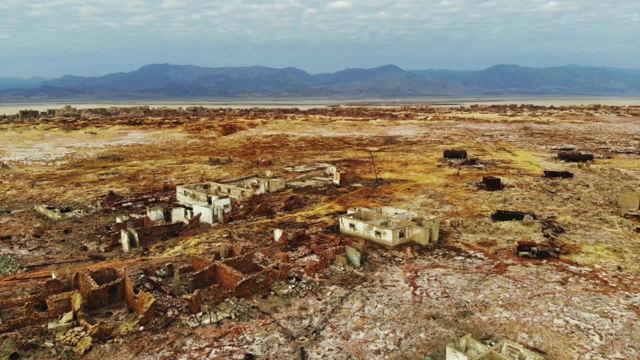 bears. In contrast, the village of Dalal Ethiopia can reach temperatures of 145 degrees Fahrenheit, And most of it sits atop an active ocean. The population of Dalal Ethiopia is about 1,000 people, And most of it sits atop an active ocean, And most of it sits atop an active 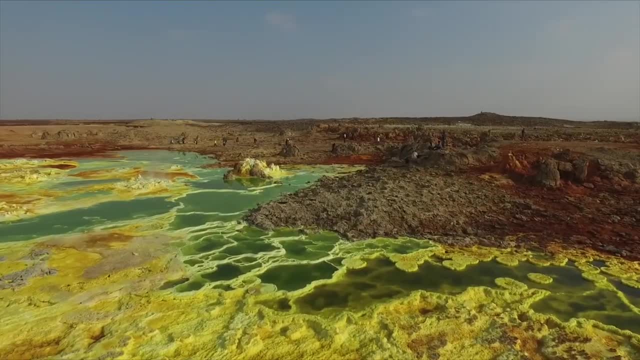 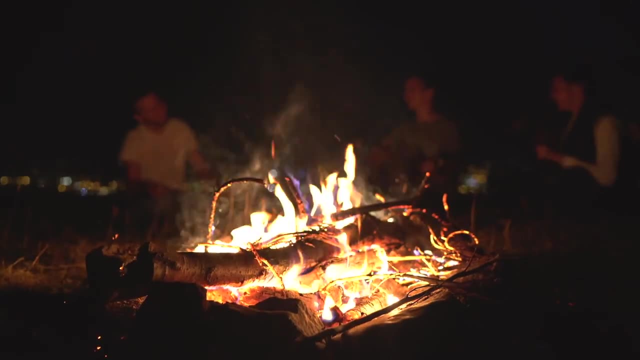 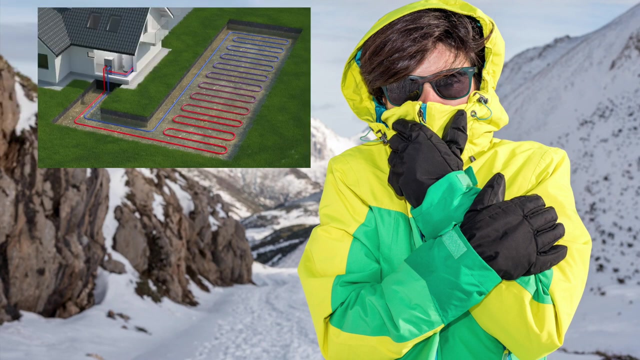 volcano. The town is abandoned now, but people still go to Dalal to gather salt from volcanic pools. These examples show that humanity has found ways to adapt to the environment to make living there possible. The people of Svalbard have insulated clothing, geothermal heat and a mandatory town law. 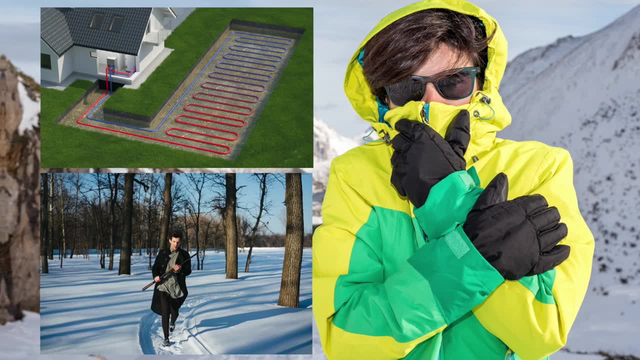 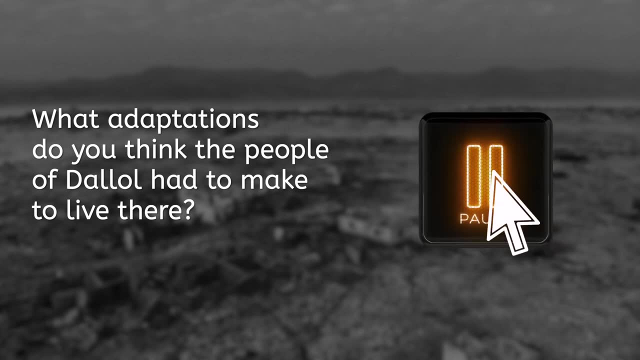 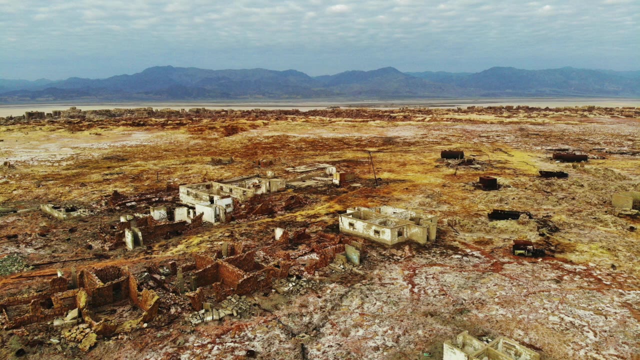 to carry a firearm for protection from the wildlife. What adaptations do you think the people of Dalal had to make to live there? Make a prediction in your lesson guide, Thank you. They crafted houses which reflect heat, wore different clothing and shoes and gathered. 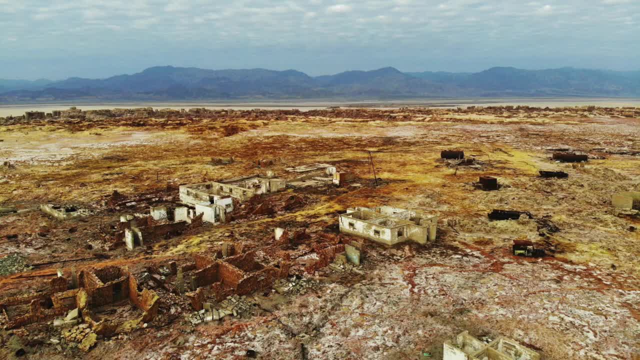 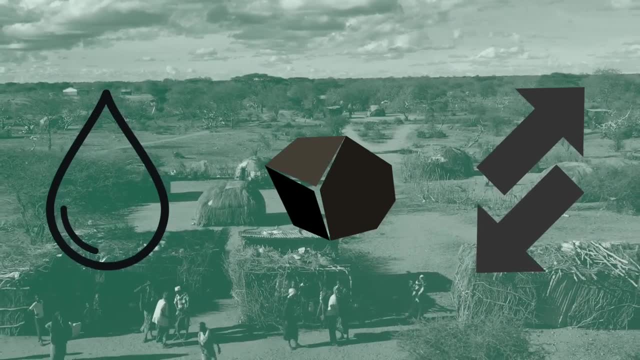 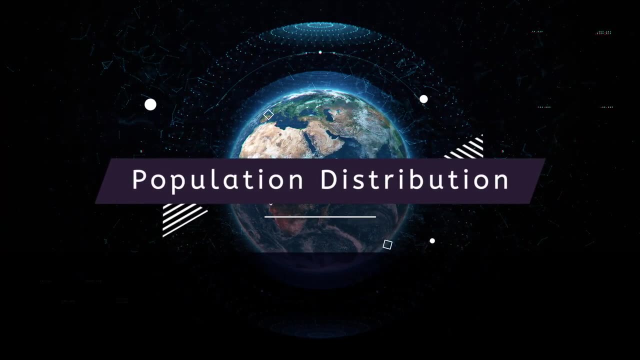 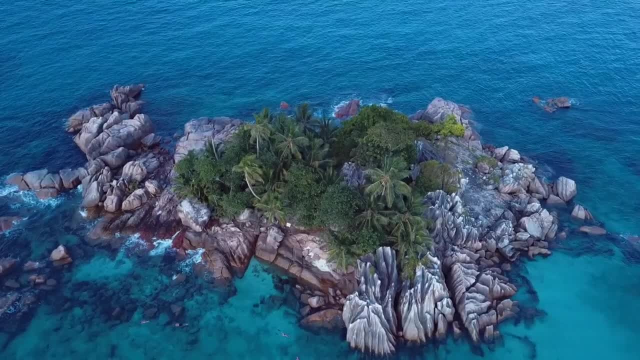 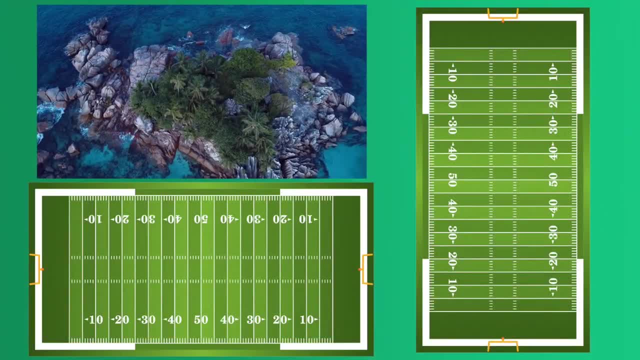 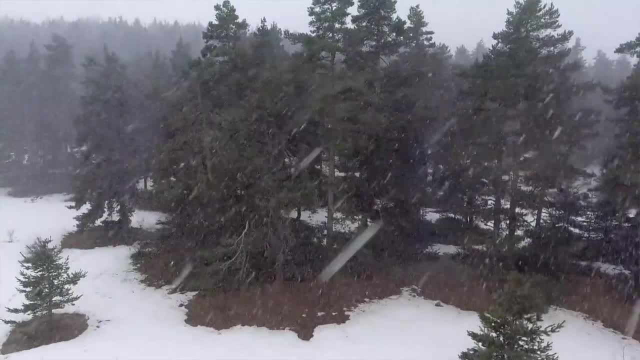 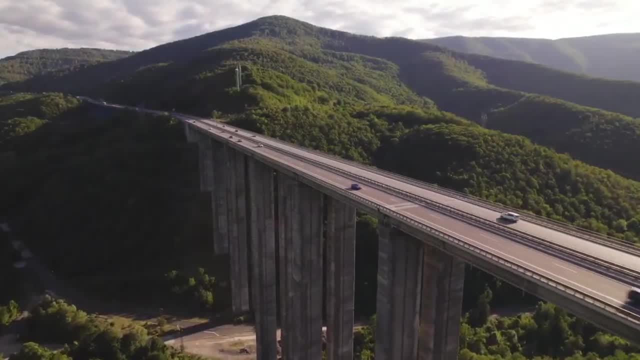 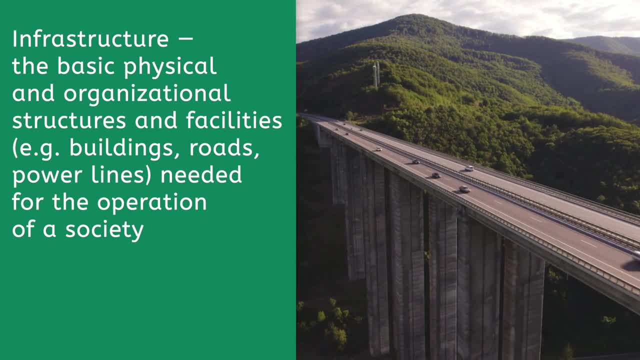 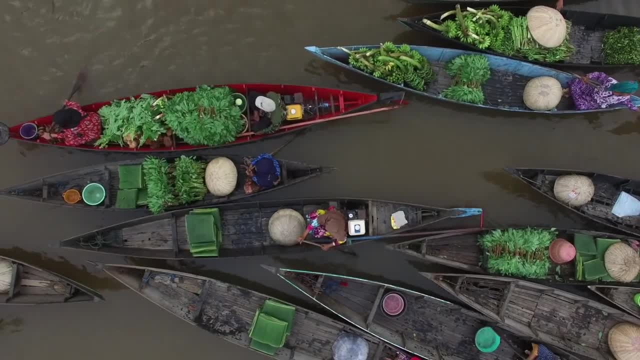 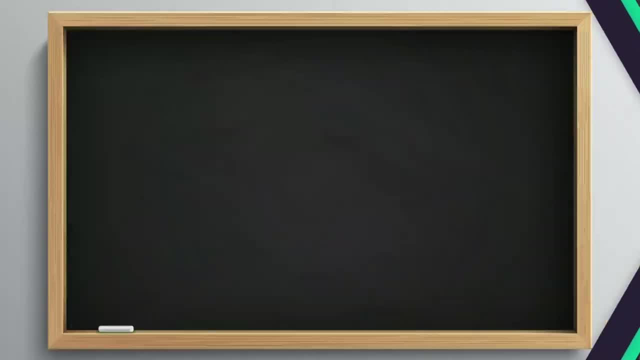 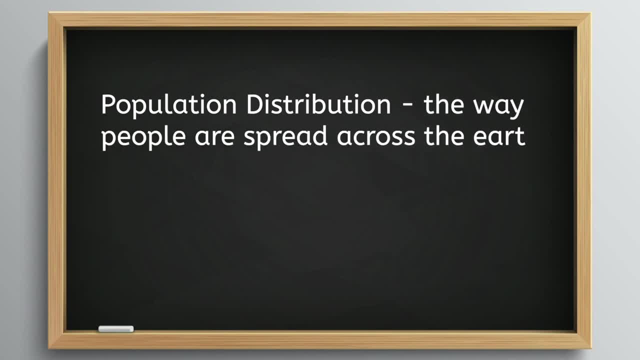 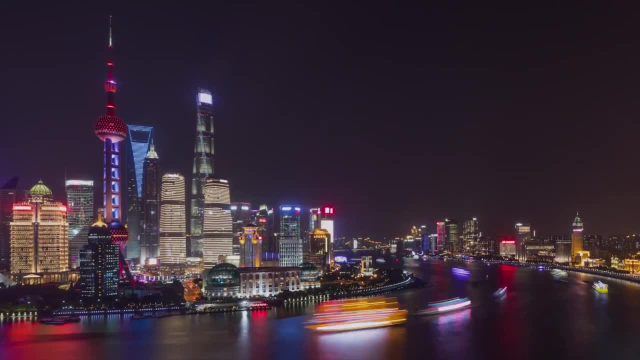 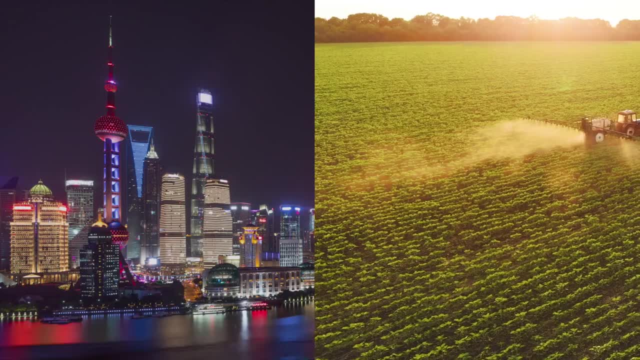 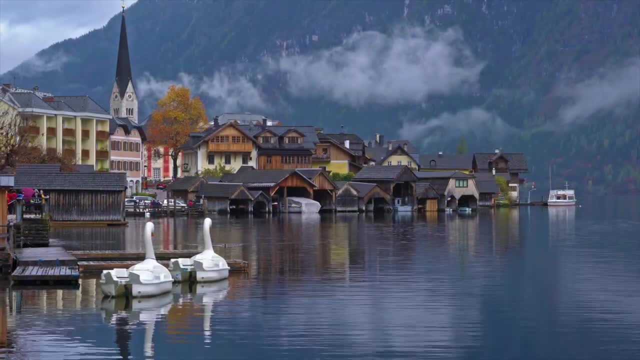 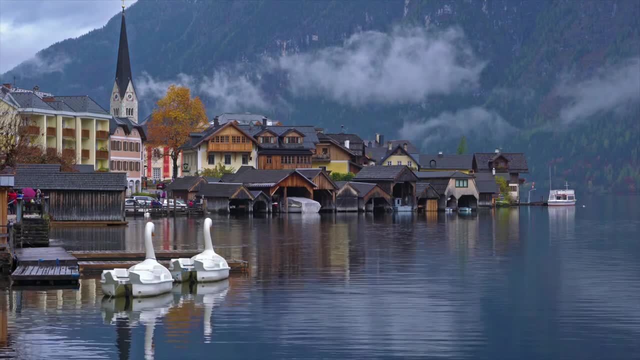 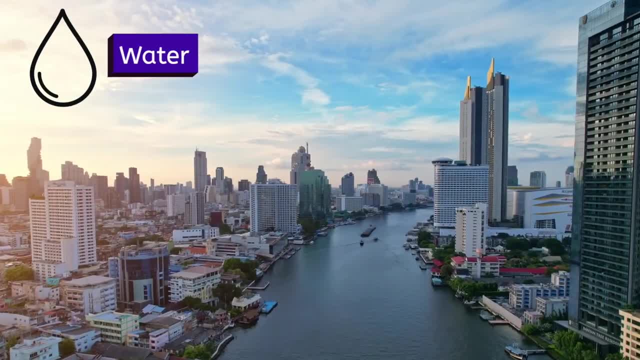 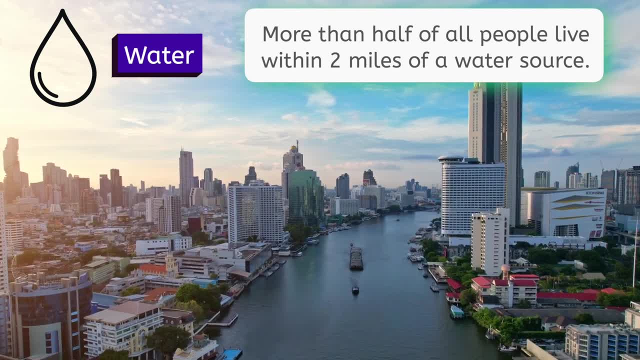 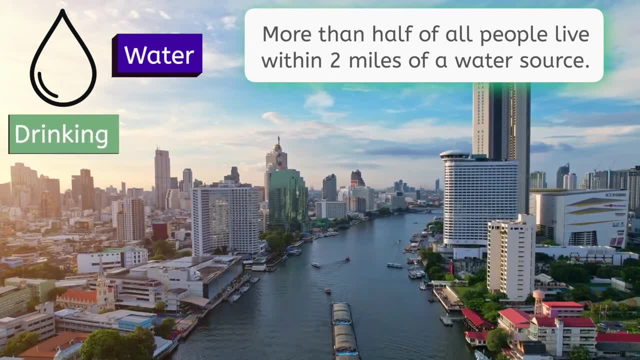 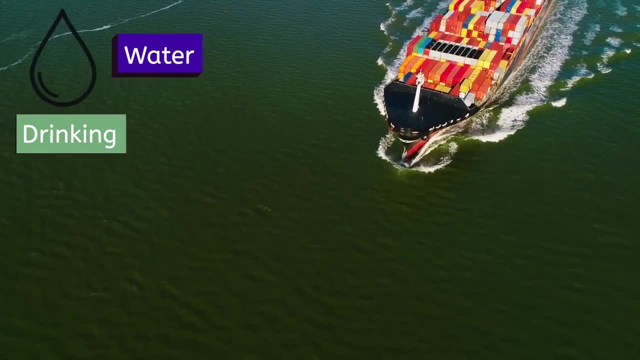 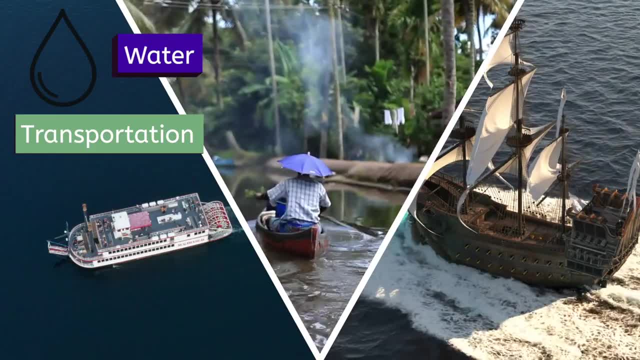 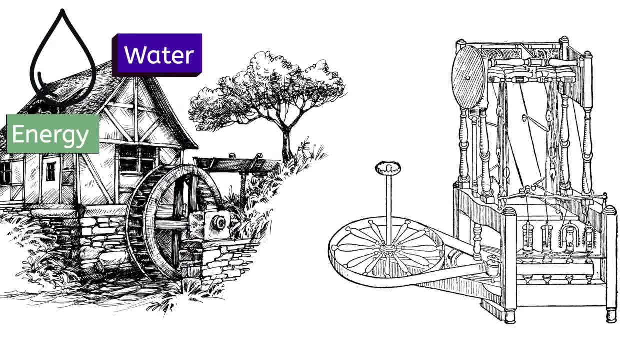 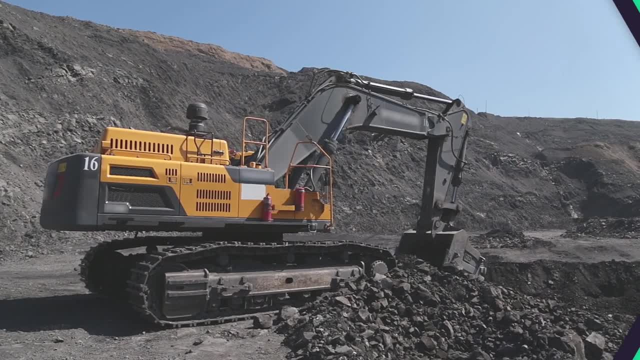 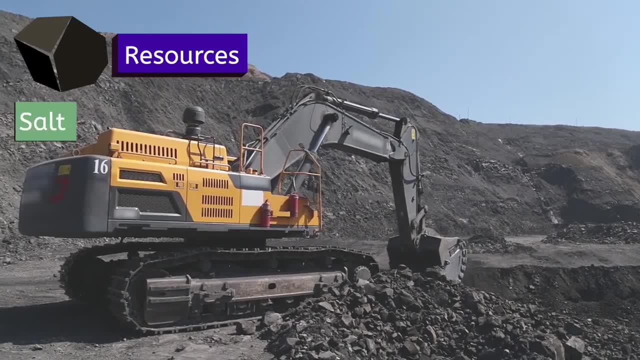 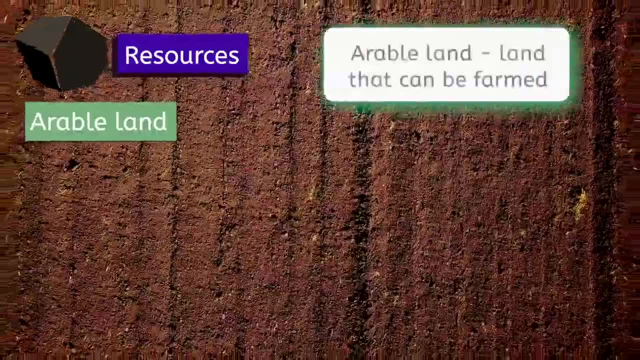 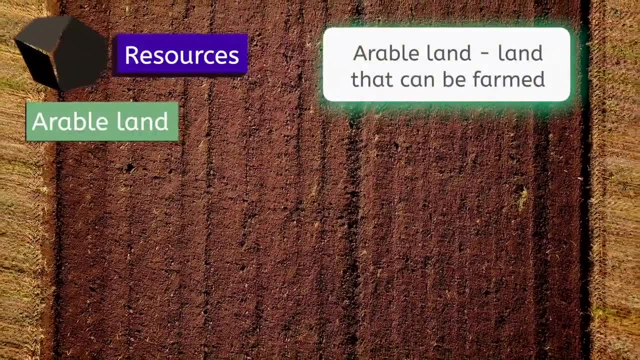 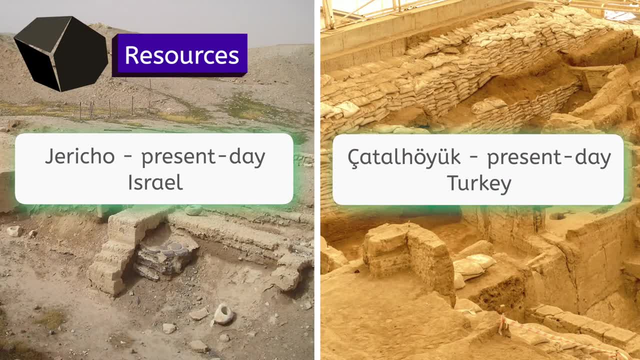 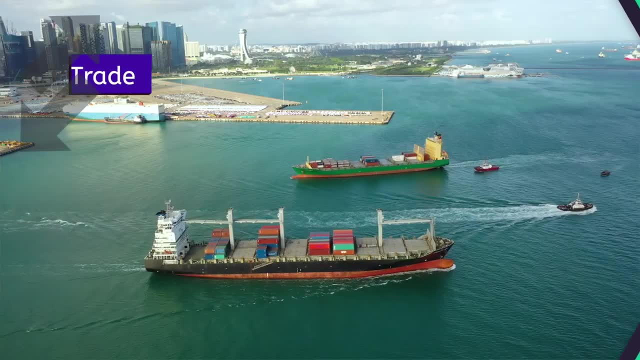 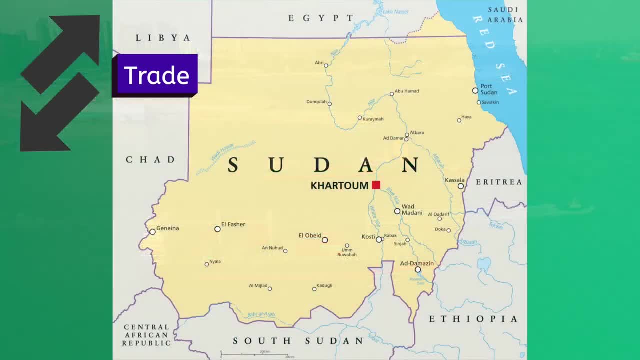 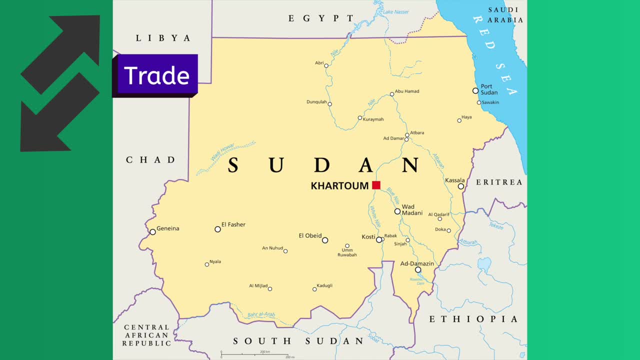 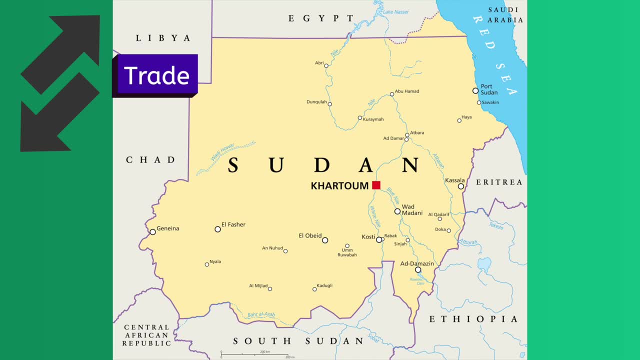 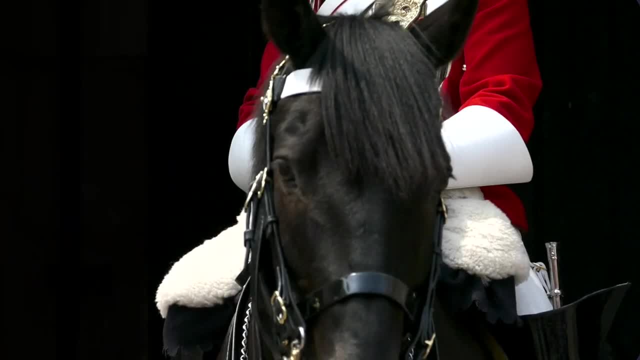 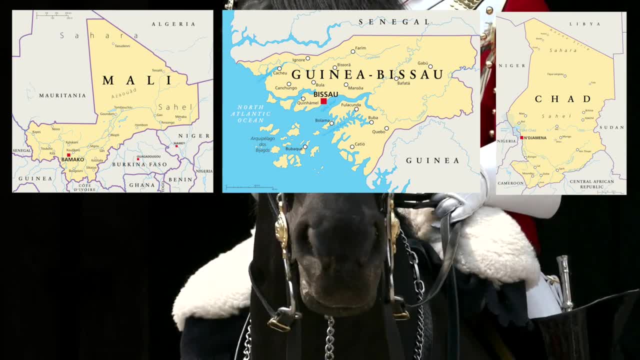 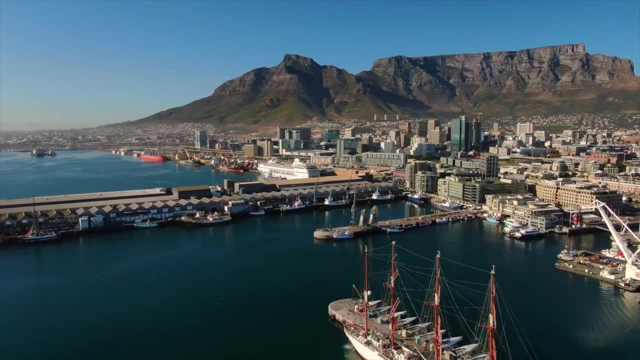 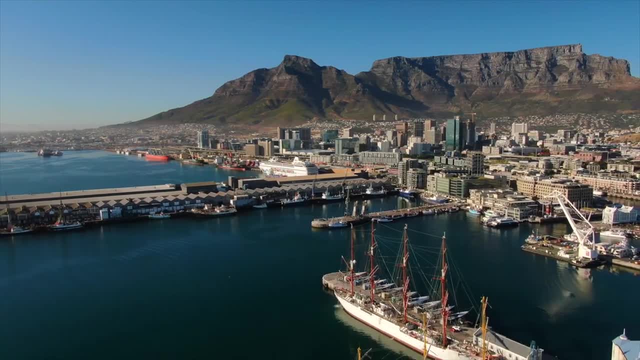 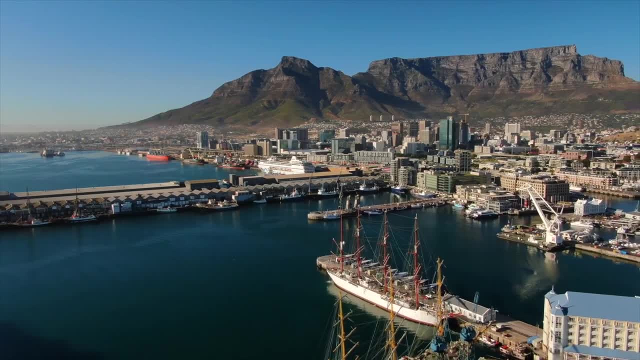 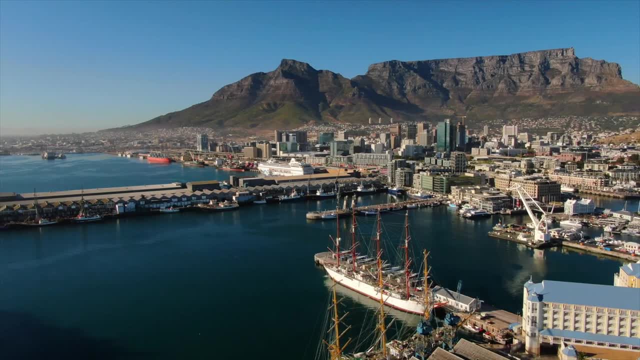 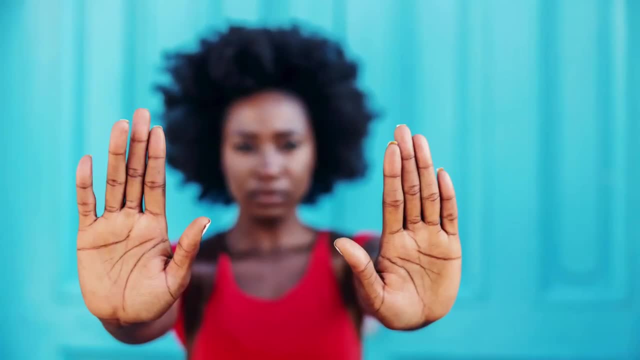 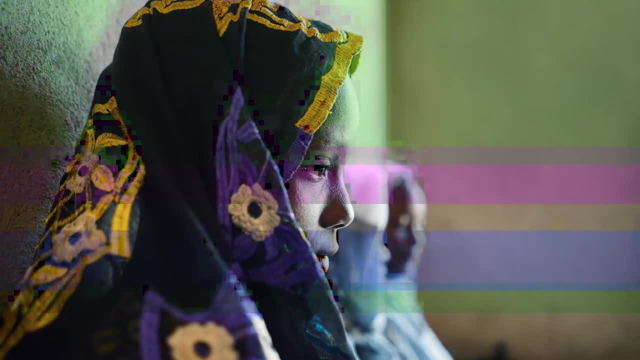 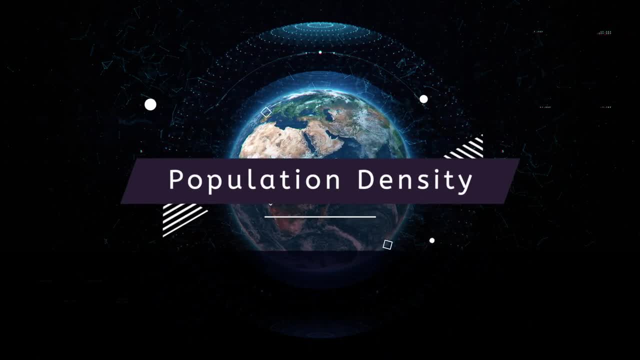 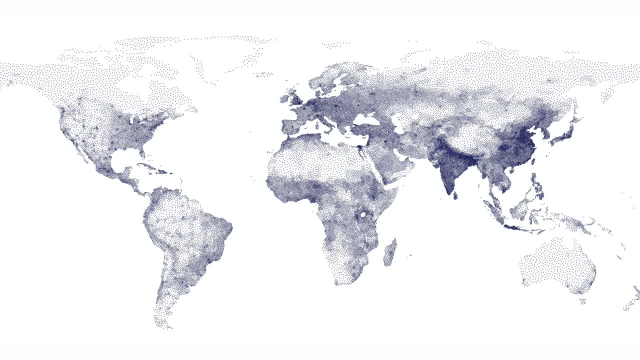 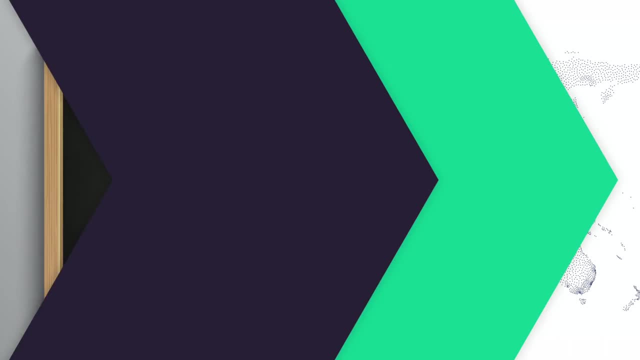 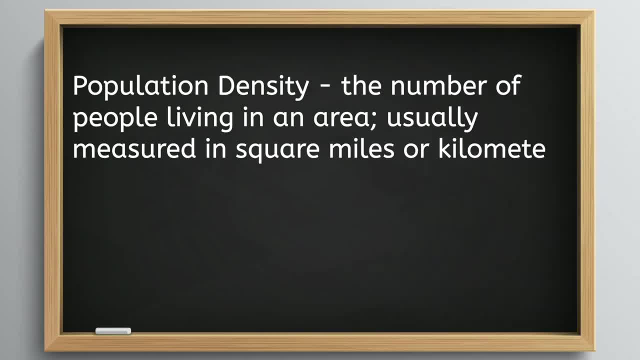 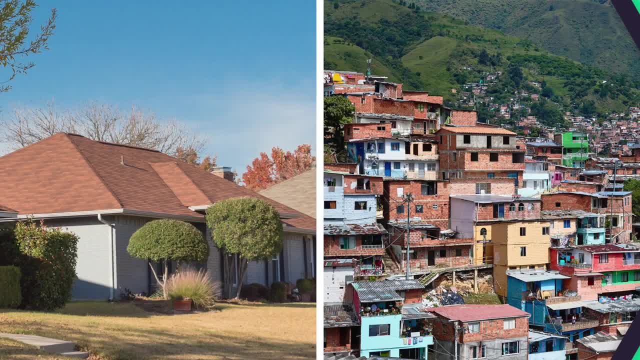 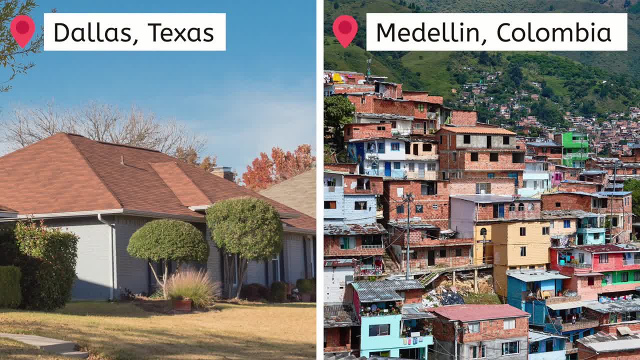 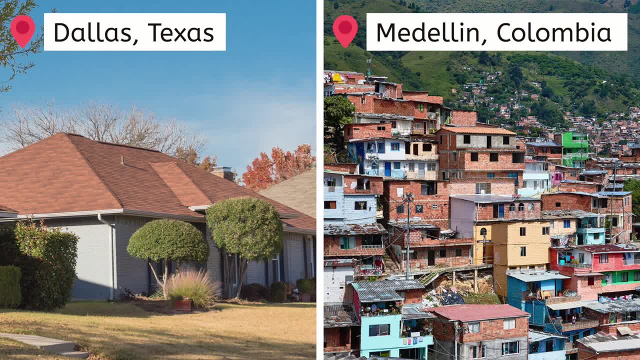 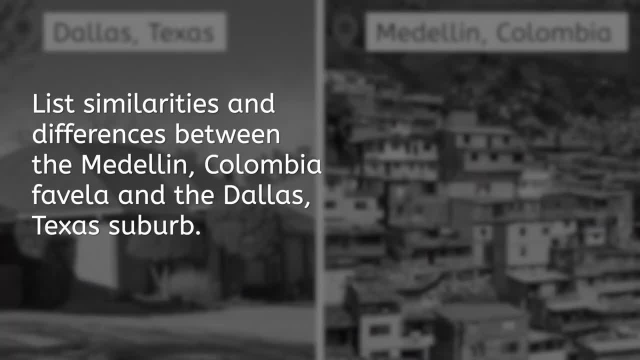 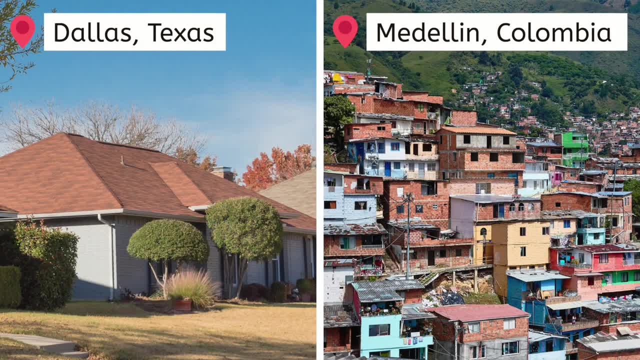 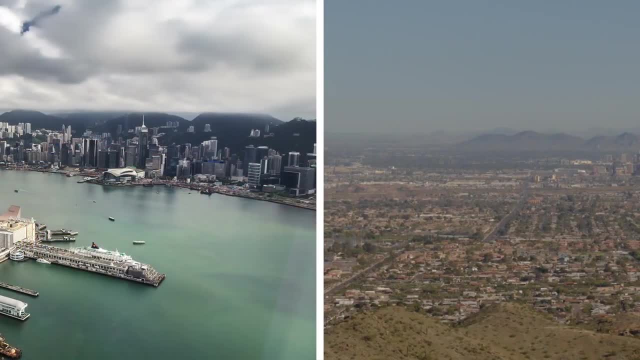 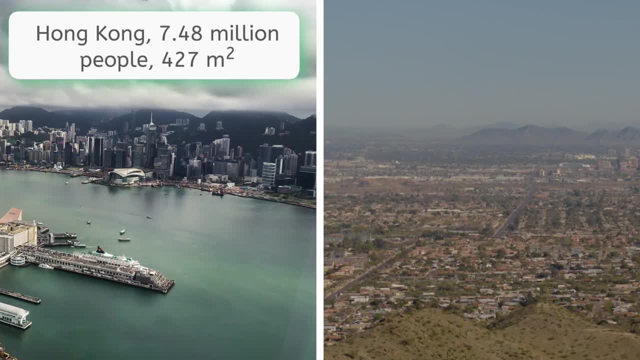 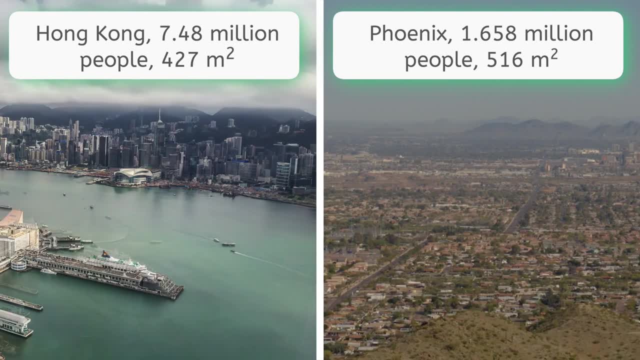 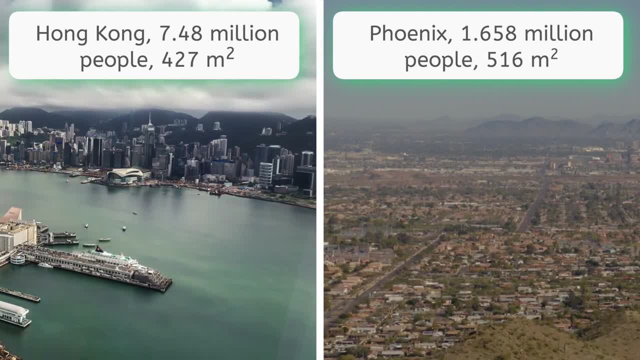 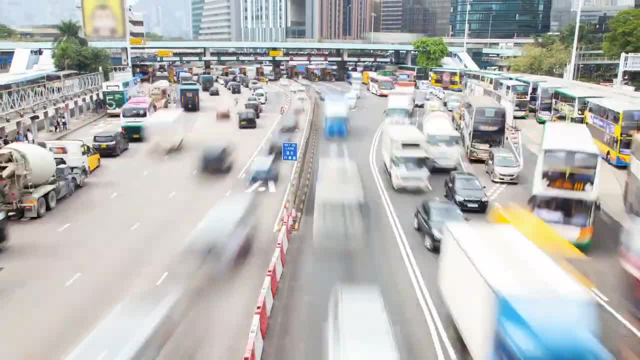 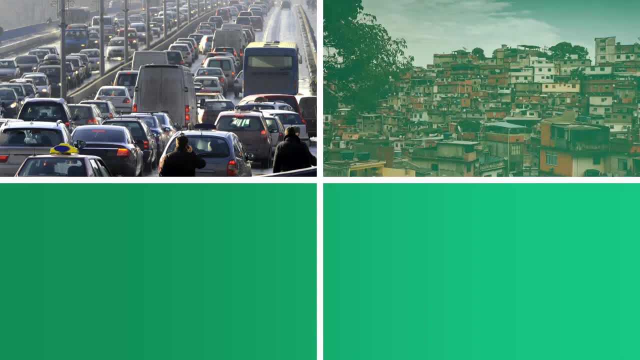 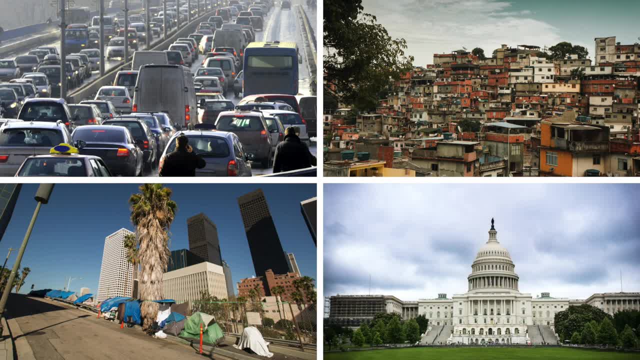 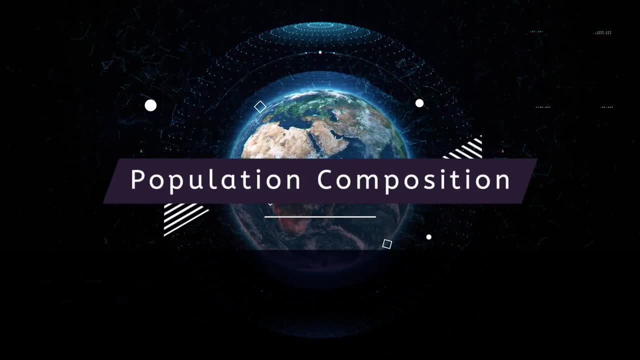 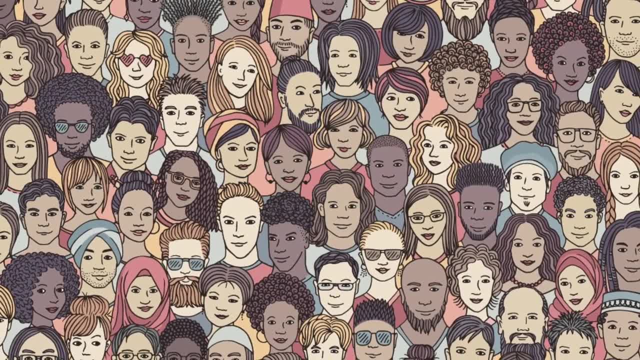 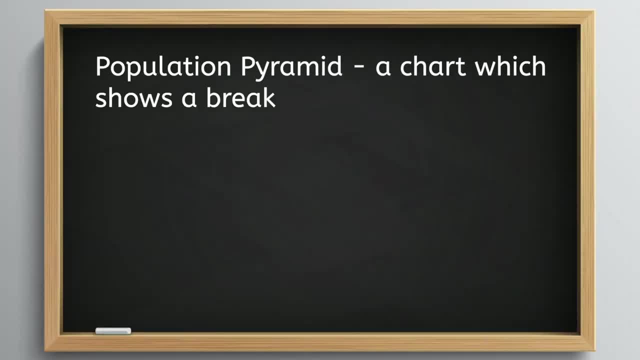 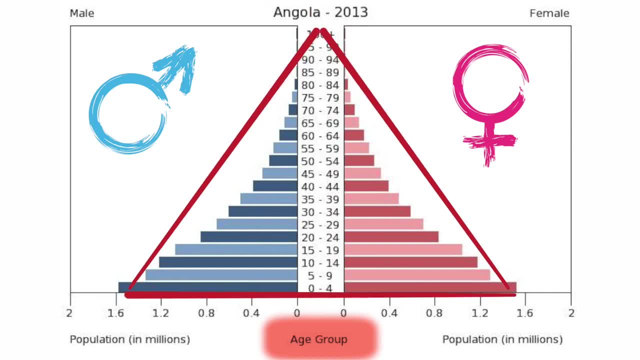 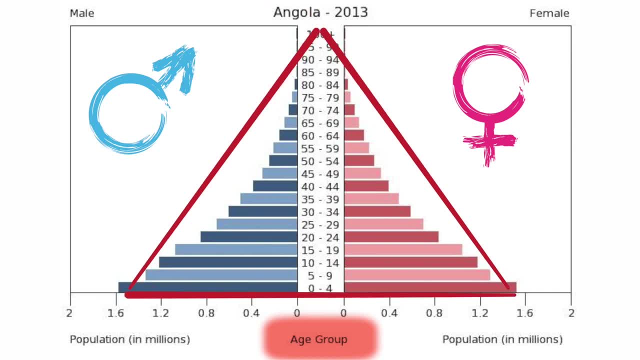 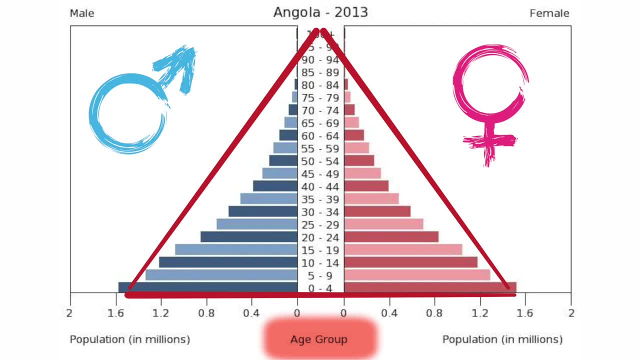 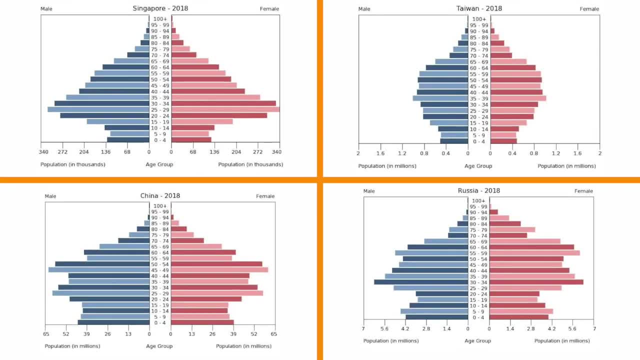 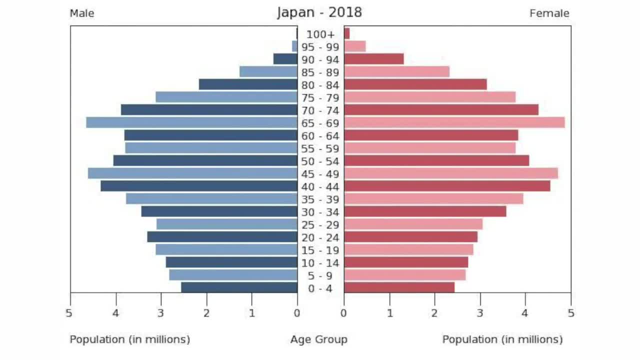 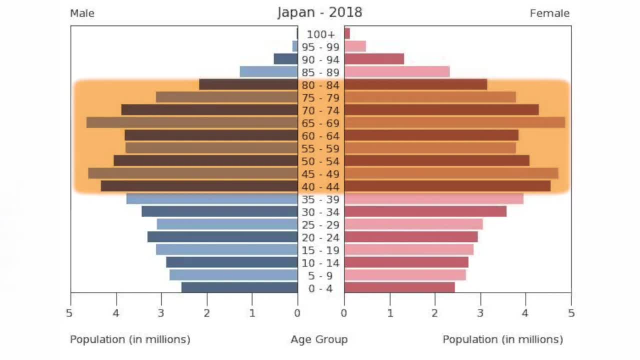 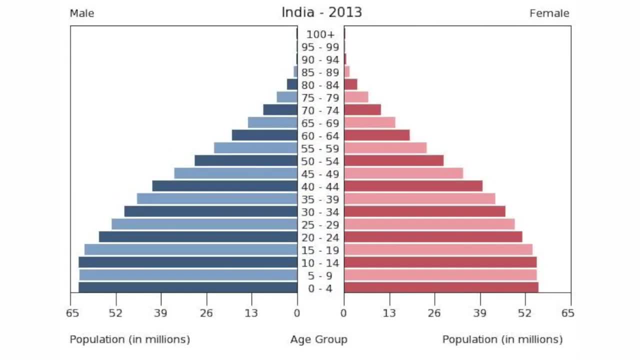 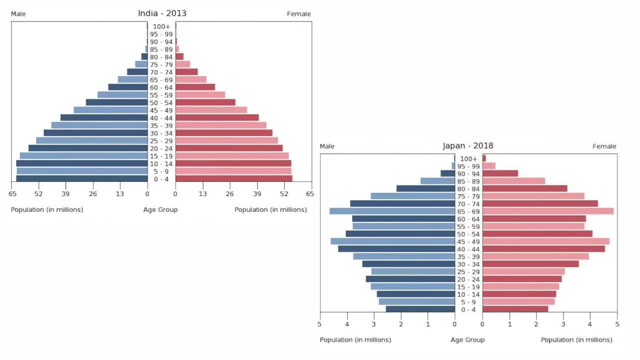 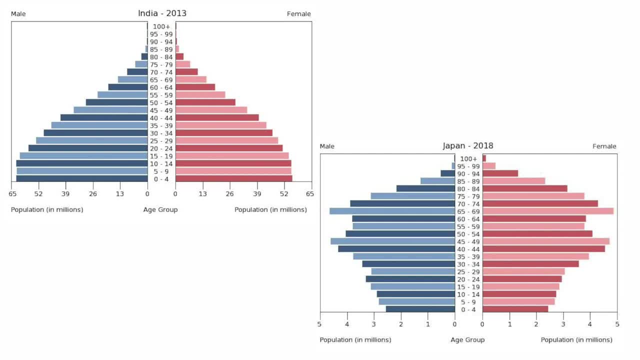 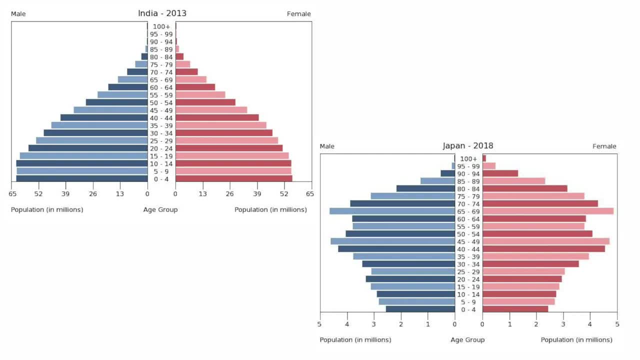 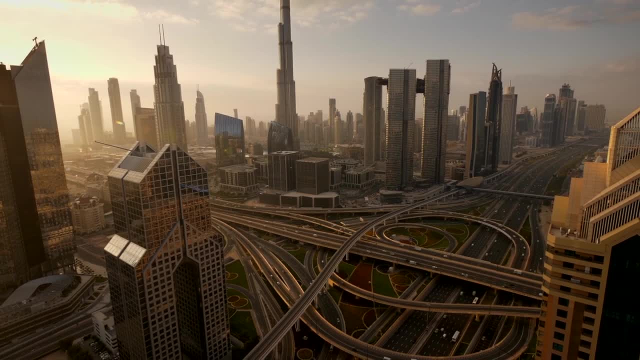 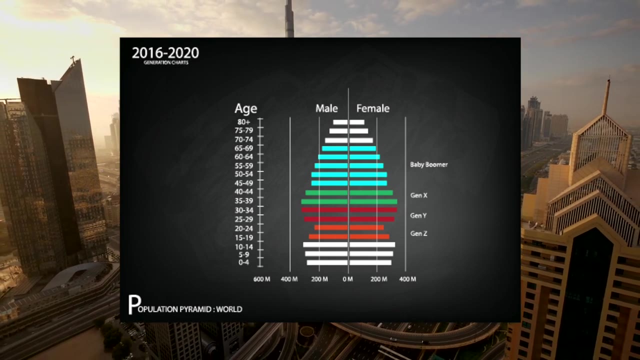 is under 35, so my bet is on Japanese voters. As we continue our study of geography, be mindful of population indicators, as it can give the geographer a powerful set of data when evaluating space and place around the world. How was your town settled and how much has it grown? 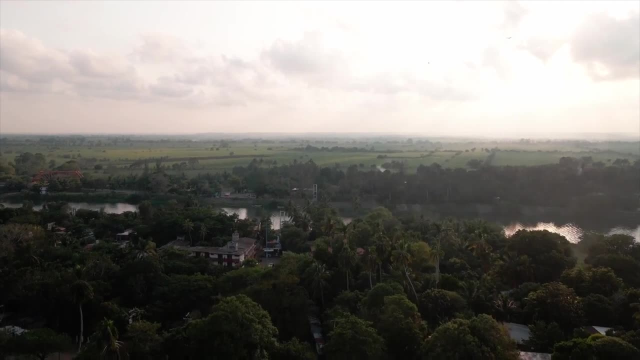 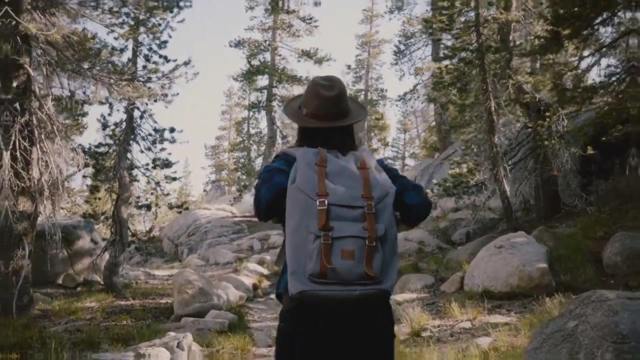 Who lives there? What resources does it have to fuel its economy? These are just a few questions you can ask to help make the world around you come alive. Remember to ask questions, be curious and, until next time, keep exploring. 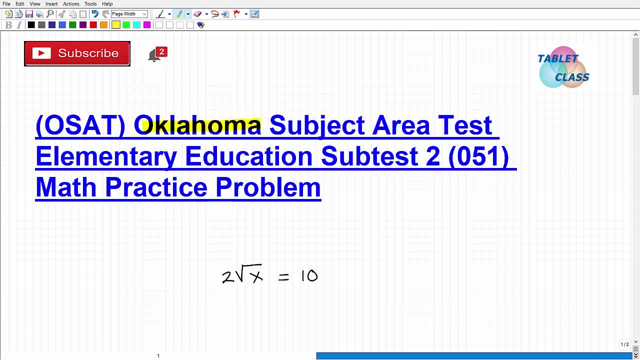 Okay, let's talk about the Oklahoma subject area test and the specific OSAT test we're going to be talking about is the elementary education And, as part of that particular test, we're going to be talking about the subtest too, And there is the test code. So very specific topic we're going to be discussing in this brief video And if you're watching this video, I assume you are preparing to be an elementary education teacher.